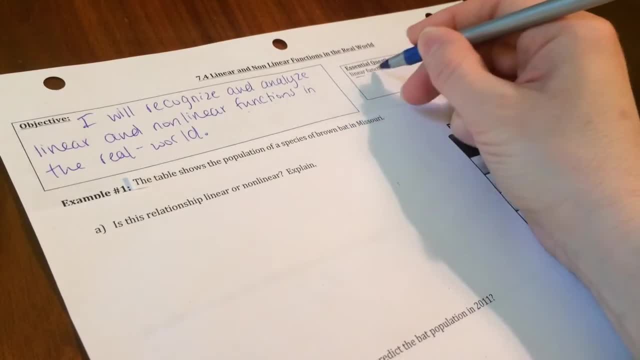 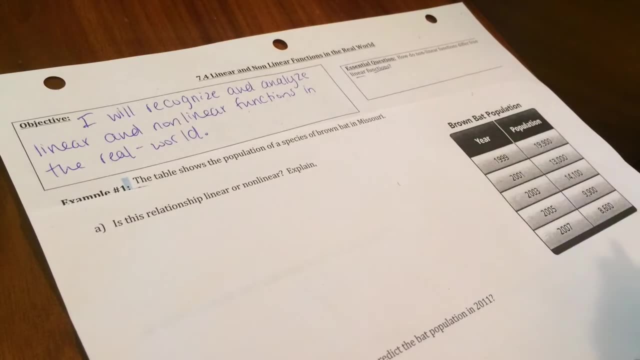 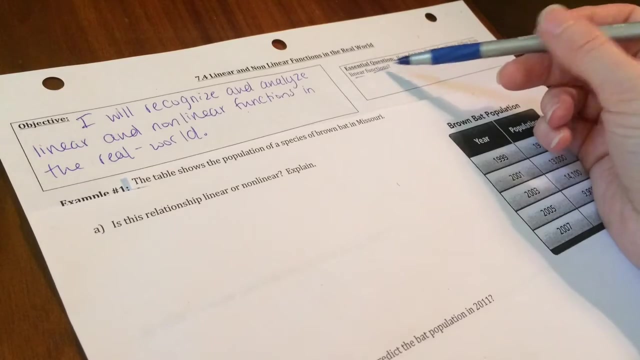 Okay, and we learned already that linear functions, when you're given a graph, are a straight line- Okay, they model a straight line. Nonlinear functions are not straight lines- Okay, and linear functions have to have a constant rate of change. 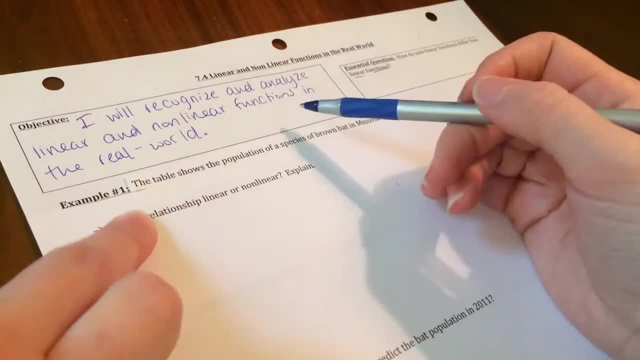 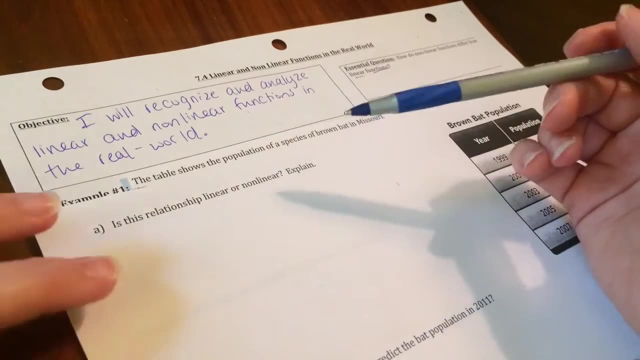 So let's look at example number one. It says the table shows the population of The population of species of brown bat in Missouri. Is this relationship linear or nonlinear? Explain, And why can't you use this table to predict the bat population in 2011?? 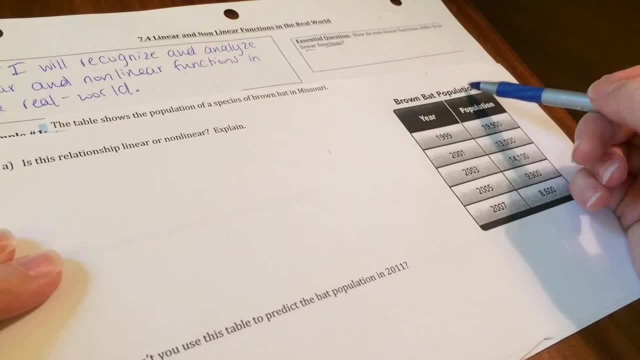 So let's look over here at the table brown bat population- They said it was in Missouri. It says year: 1999,, 2001,, 2003,, 2005,, 2007.. And then it gives you the populations of each year. 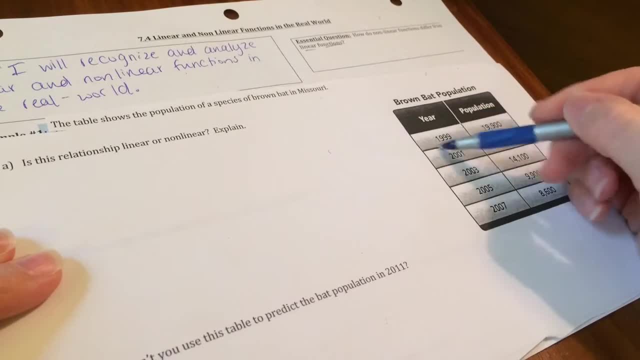 It looks like from this table, the first year they have down is 1999.. So that was the year that they started recording the population of the bats, And it looks like they went all the way up to 2007.. Okay, so they recorded them. 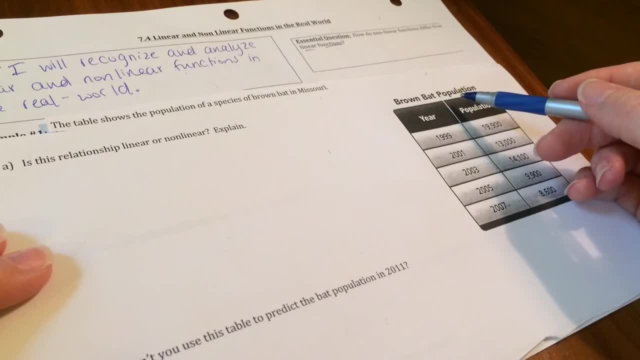 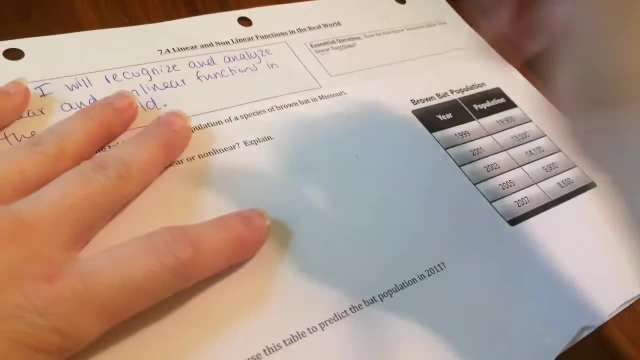 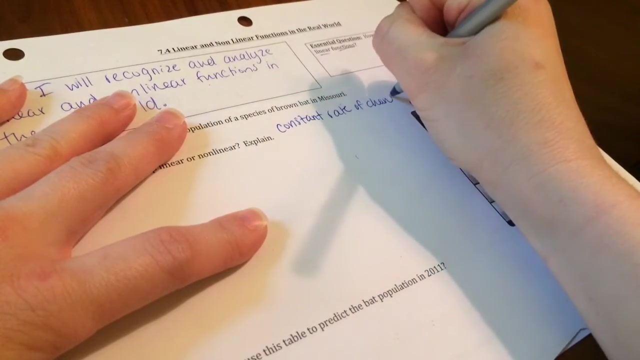 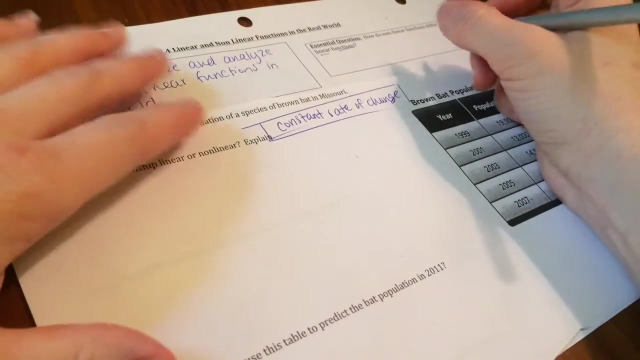 And let's see we're trying to figure out. first, is this relationship linear or nonlinear? Remember, a linear function has to have write this down: a constant rate of change. A constant rate of change, All right, and remember when you're given a table. 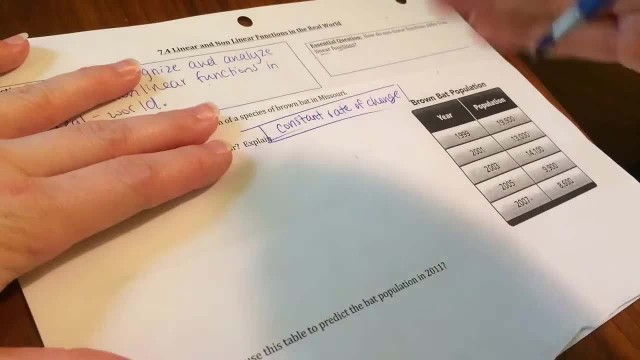 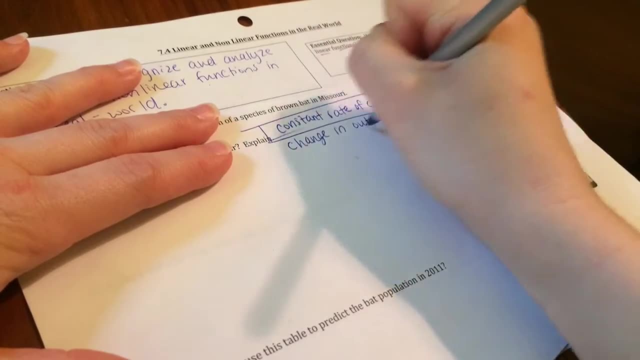 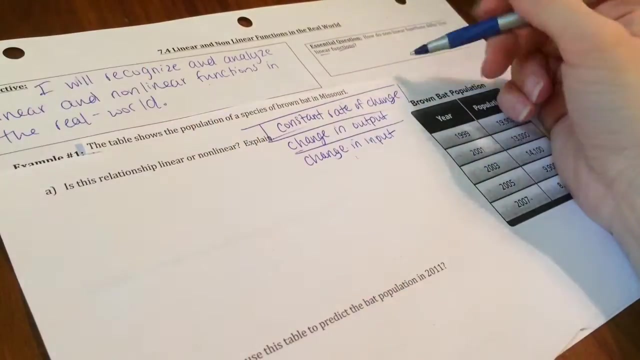 the way that you know if something has a constant or the way that you know what the rate of change is is. you have to take the change in output and put it over the change in input. All right, just like the output is your y values. 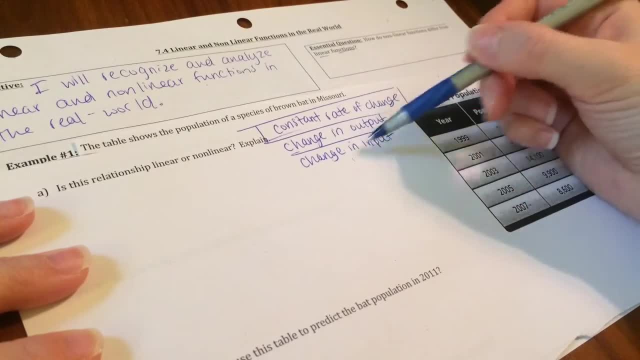 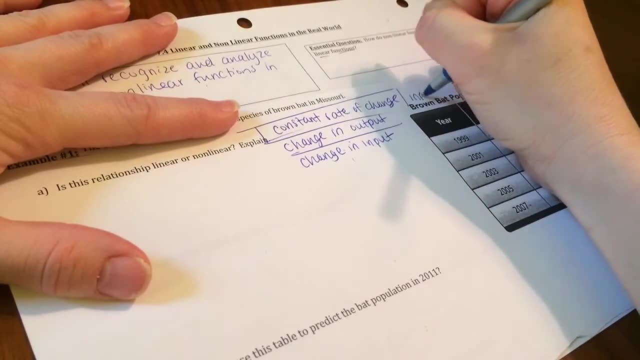 And the input is your x values. It's like the rise over the run, the change in output over the change in input, Because the rate of change, remember, is like the slope. So here we have the years, or the input. that's like your x values. 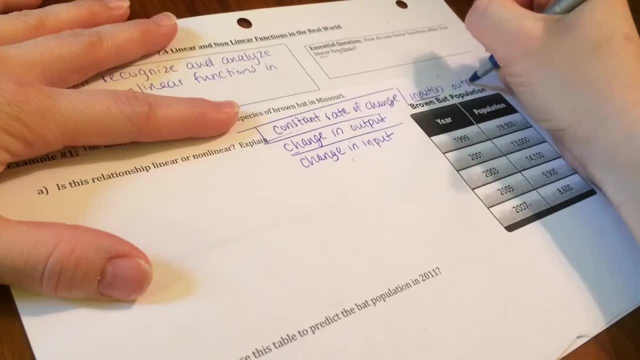 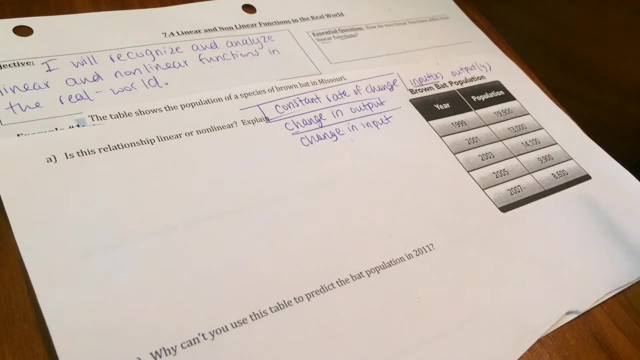 And the population is your output. Go ahead and copy this down. that is your y values. All right, because the population depends on the years. It's like the years are the cause, the population is the effect. The years happen. first time has to happen before you have a population. 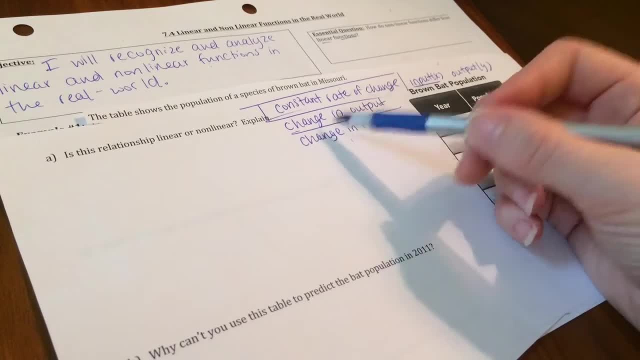 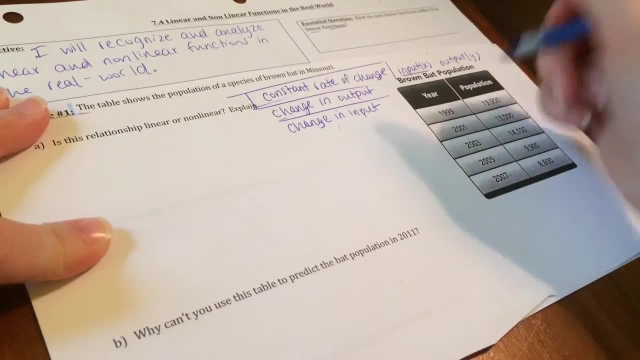 All right. so the years are the input, the population is the output. So now we have to figure out the change in output and the change in input to see if it's constant. Well, like we said, they started in 1999 and then they recorded again in 2001,. so that was two years later. 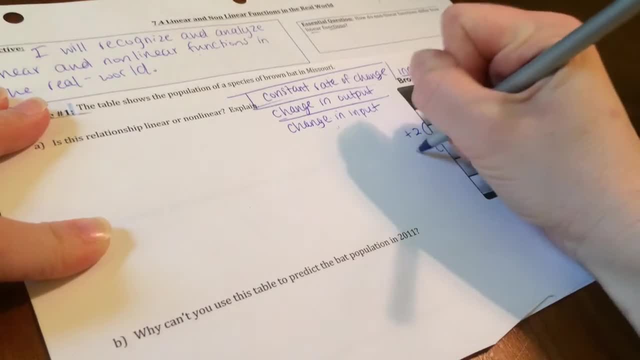 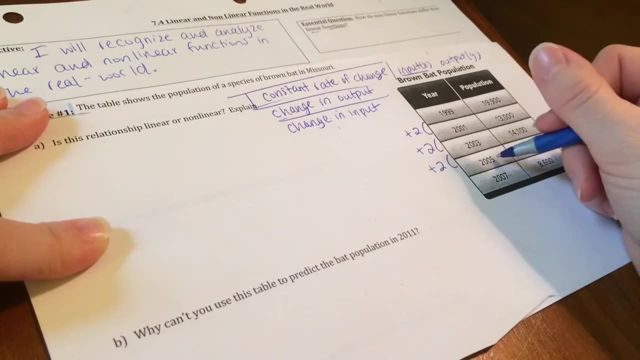 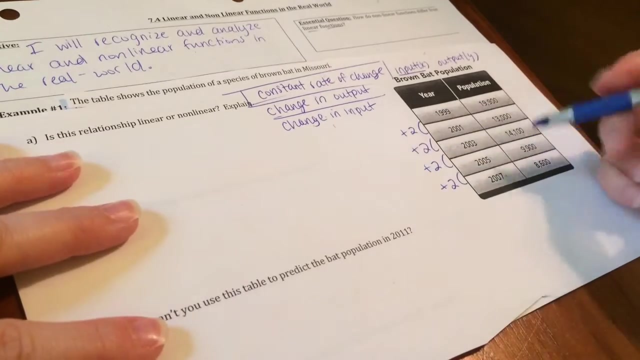 From 2001 to 2003,. you're adding on two more years: 2003 to 2005,. you're adding on two years And then 2005 to 2007, every two years. So it looks like they recorded the population every two years. 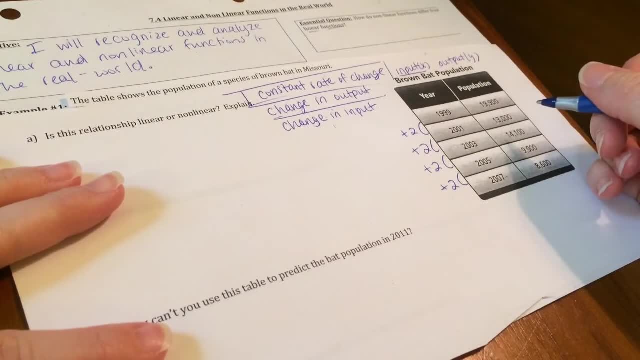 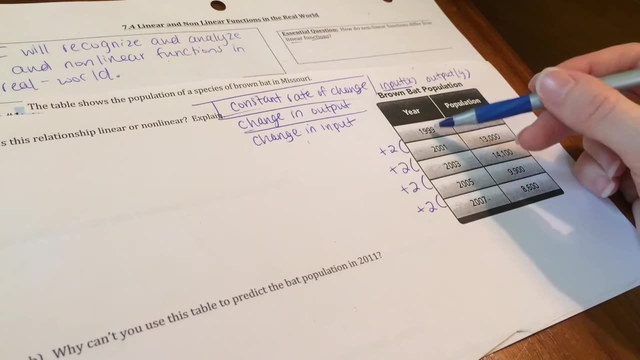 So the change in input is the same. Let's check the population now, the change in output, to see if it's the same. Notice the first recording in 1999.. It was 99. It was 19,900 bats. 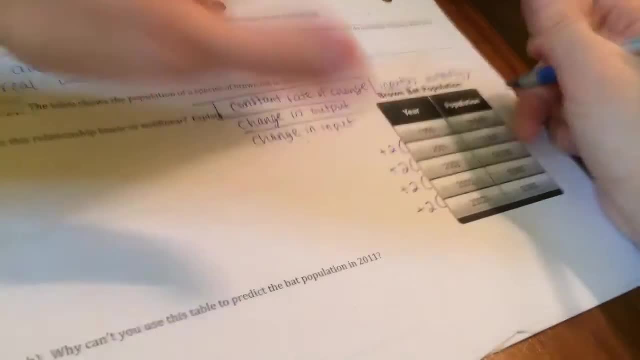 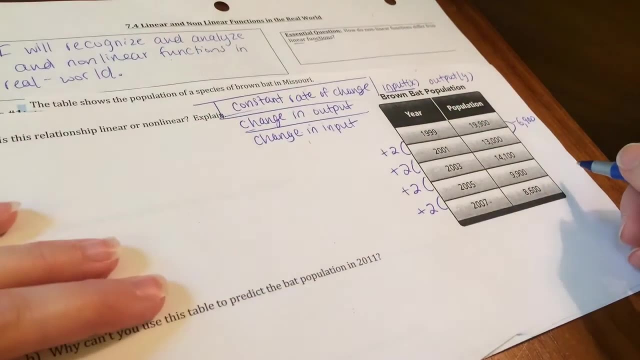 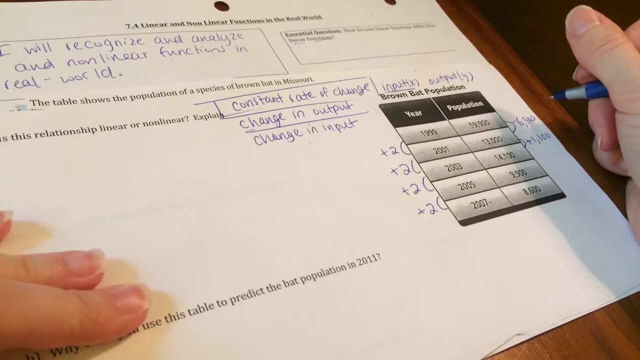 But then in 2001, it went down to 13,000.. So the change there was minus 6,900.. Then it went from 13,000 up to 14,100, which the change is 1,100 adding on. 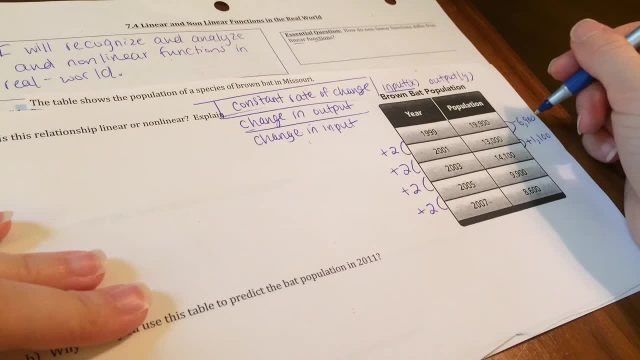 So here the change in output is already not constant. First the bat population went down 6,900.. Then it went back up 1,100.. Then from 14,100 to 9,900, the change there is minus 4,200. 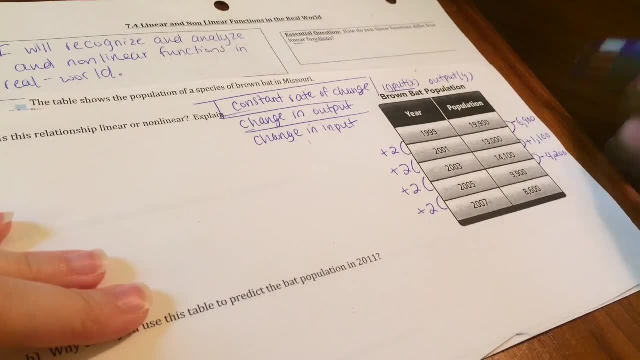 So here the bat population went down again, And then, from 9,900 to 8,600, the bat population went down again Again, It went down 1,300.. As you can see that the change in output is not constant. 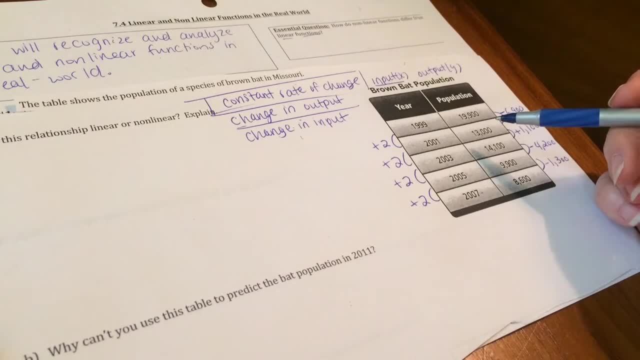 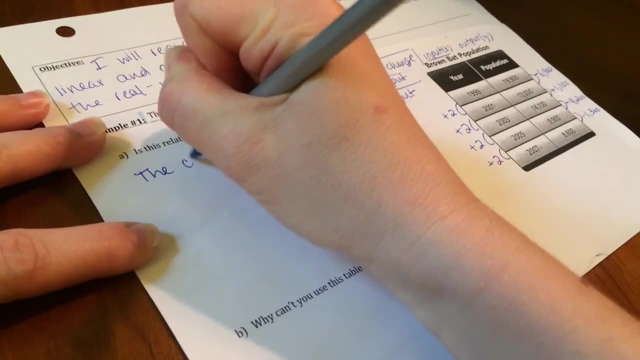 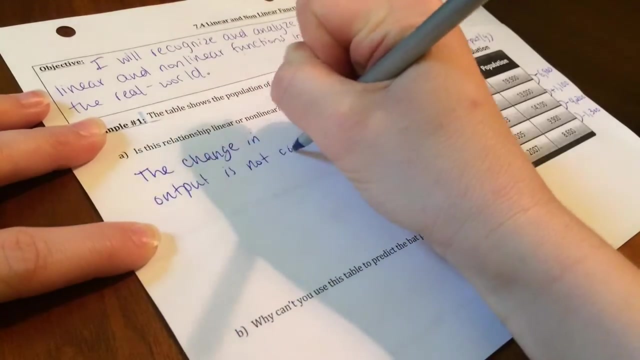 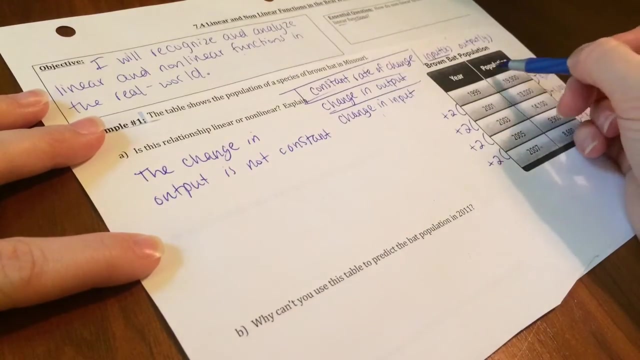 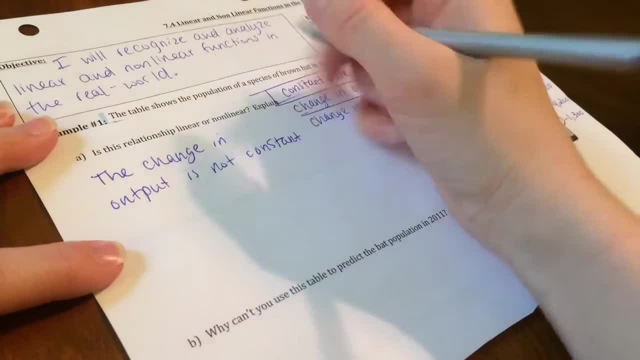 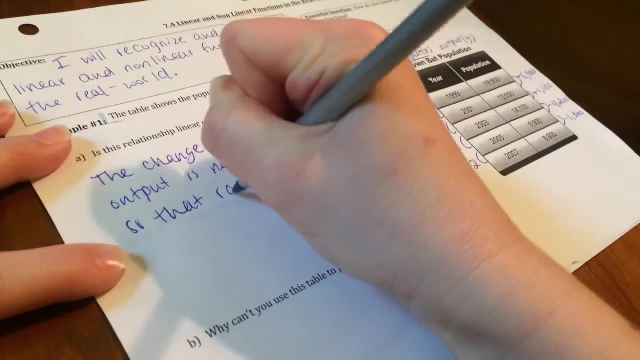 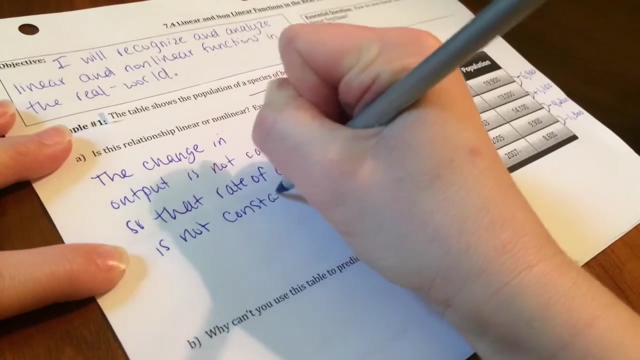 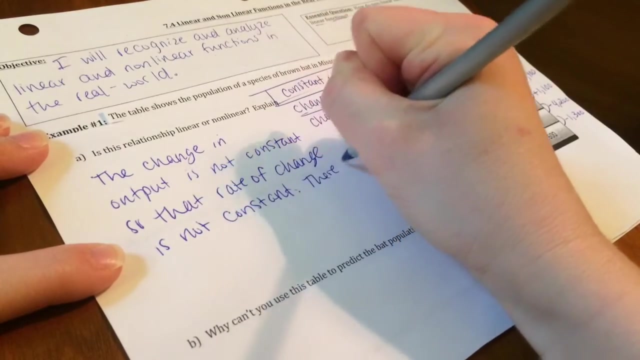 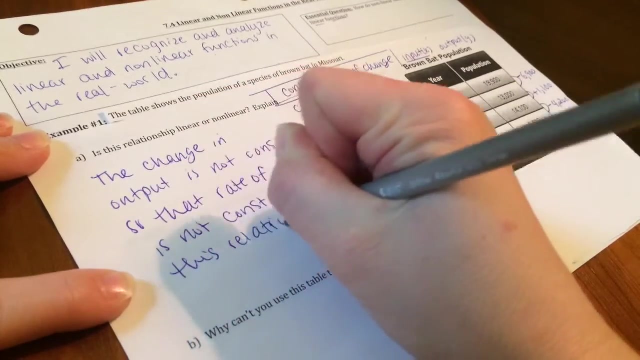 So the change in population is not constant every two years, So the rate of change is not constant. Which means to answer this: is the relationship linear or non-linear? Therefore, the relationship between years and population is non-linear. This relationship between years and population is non-linear. 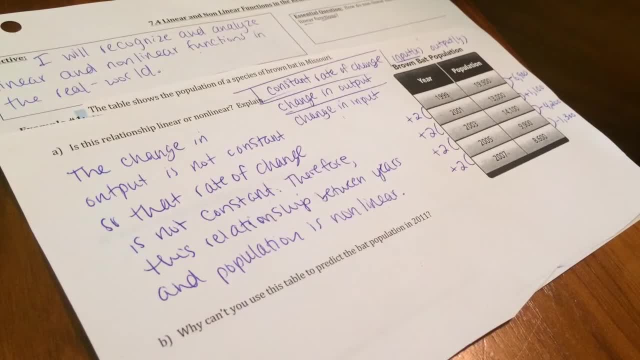 Okay, because, again, the change in population is not constant. So, to answer letter B, why can't you use this table to predict the bat population in 2011?? Well, like we said, even though the years were constant, they were recording every two. 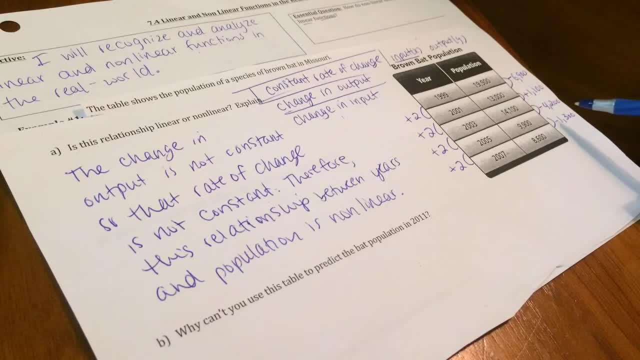 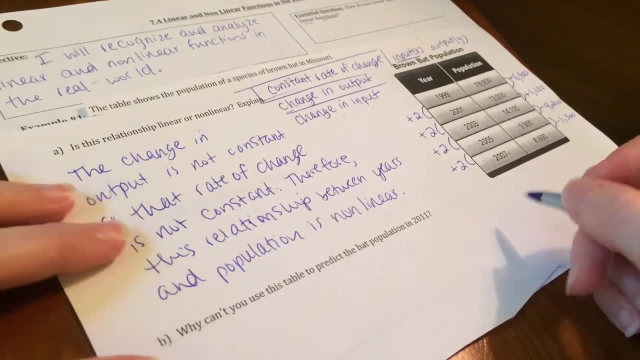 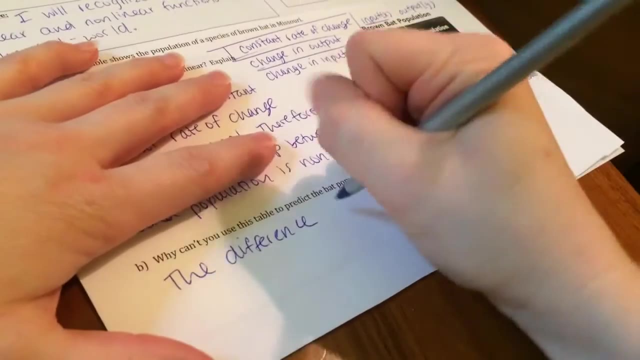 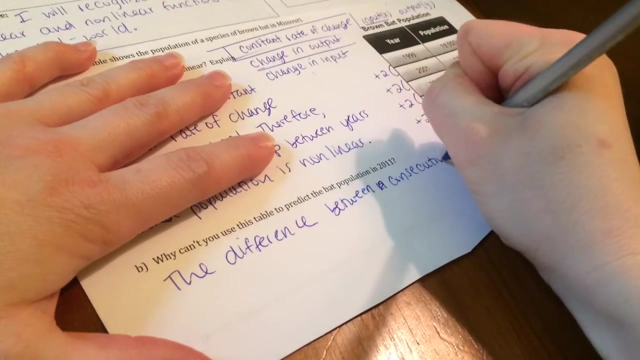 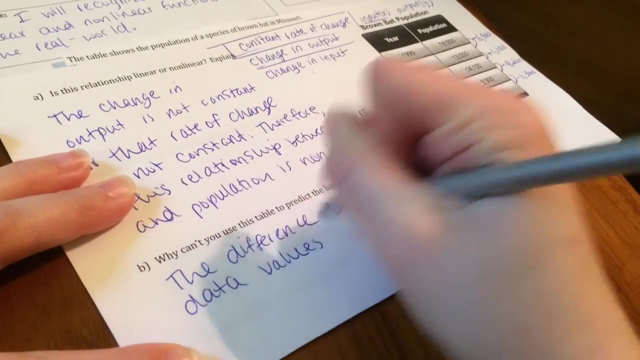 years. the population change isn't constant. There's no pattern here. So what we can say is the difference between consecutive meaning one after the other data values. right, Like they're checking it every two years. They're consecutively checking it every two years. 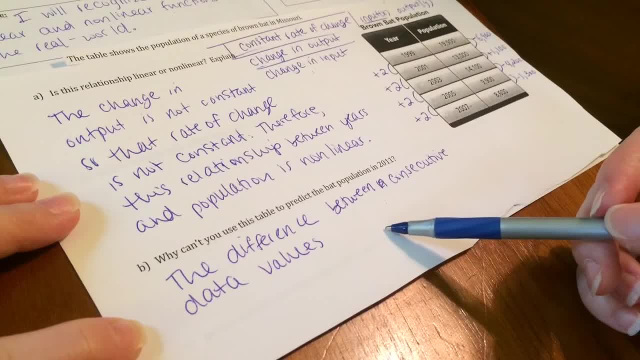 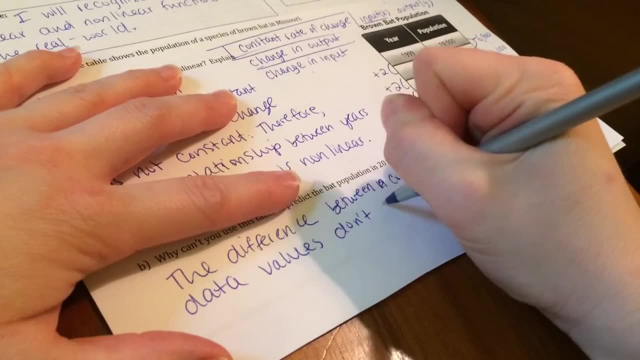 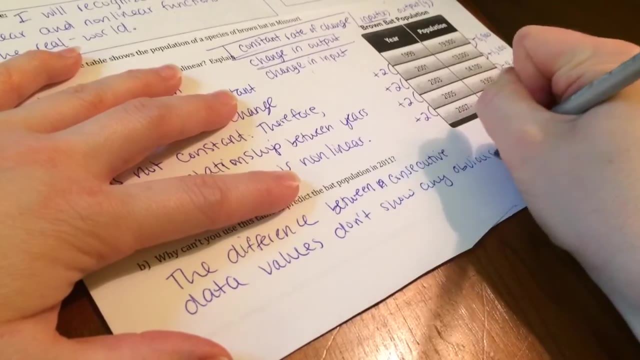 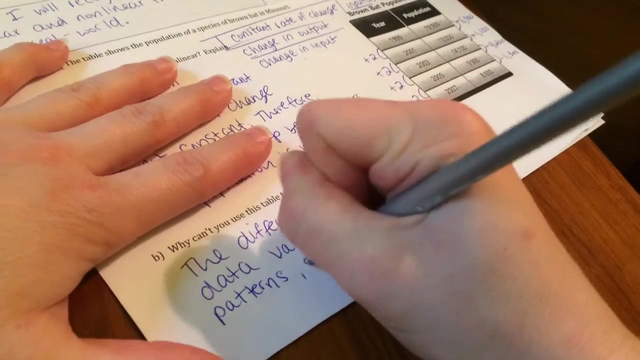 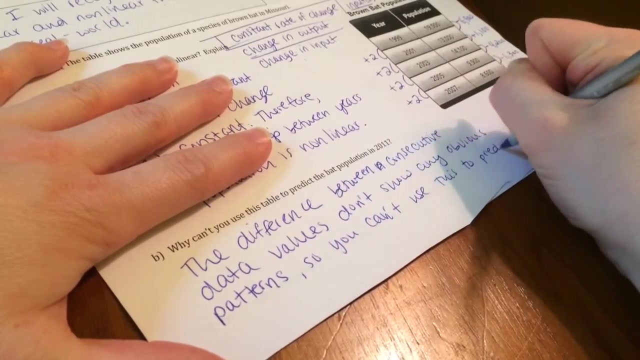 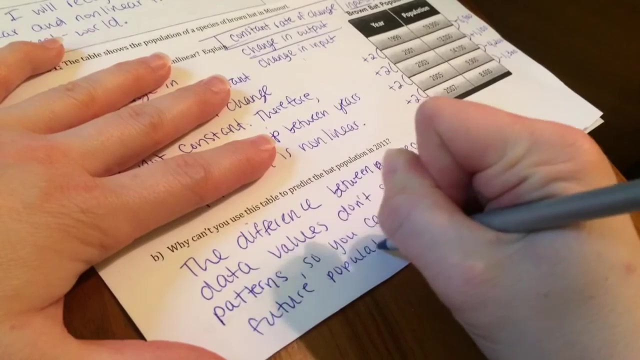 But the difference in population? No, It doesn't show. So these data values don't show any obvious patterns, right? Because it's not the same each time. So you can't use this to predict. Okay, So you can't use this to predict future bat populations. 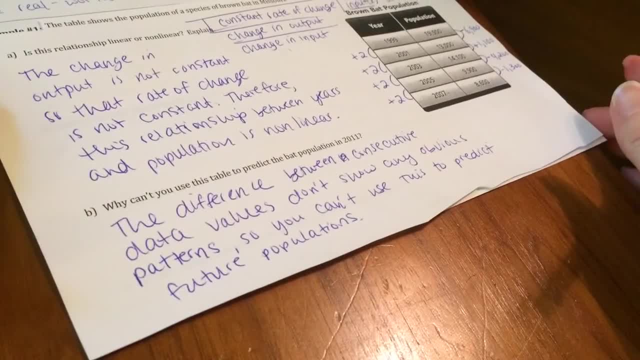 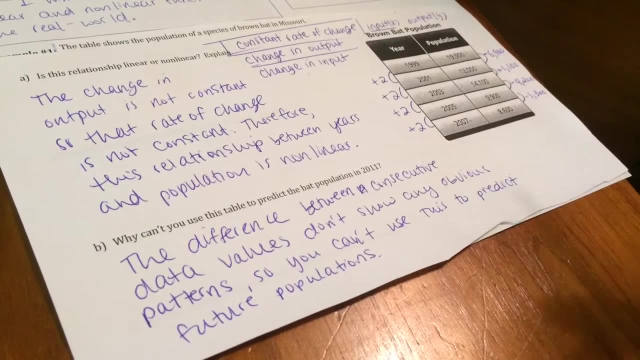 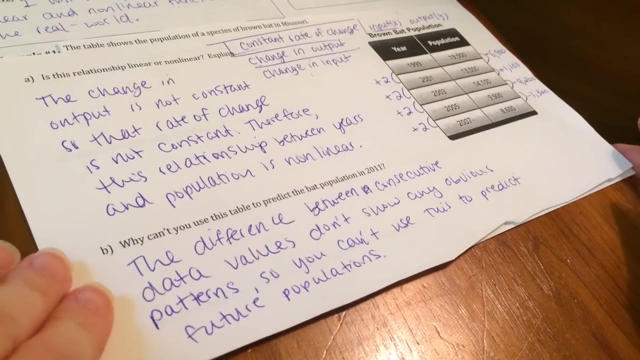 All right, Because it's not constant. there's no pattern here. You can't use this to predict the bat population. All right, After you finish copying these notes, go ahead and go on to example number two, And then you have one. And then you have one guided after that.